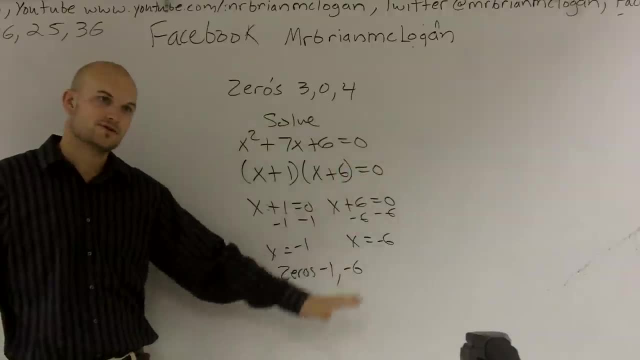 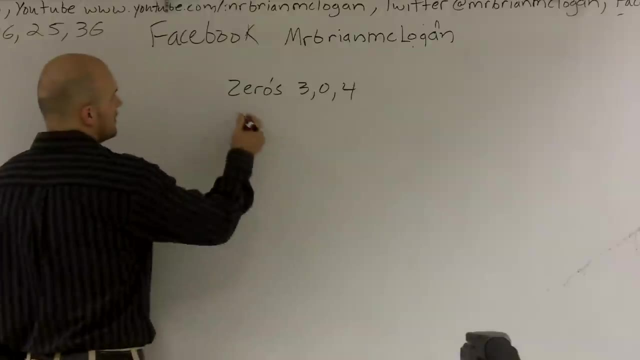 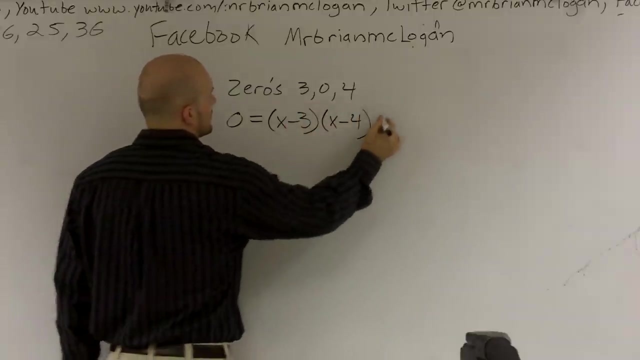 Because, remember, we write it as x plus 6 equals 0.. So we're just going to work backwards. So therefore, if I want to write my zeros as a list of linear factors, I'll write: 0 equals x minus 3, x minus 4, and x minus 0. 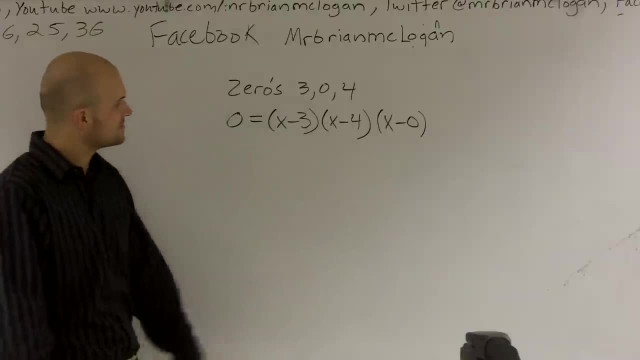 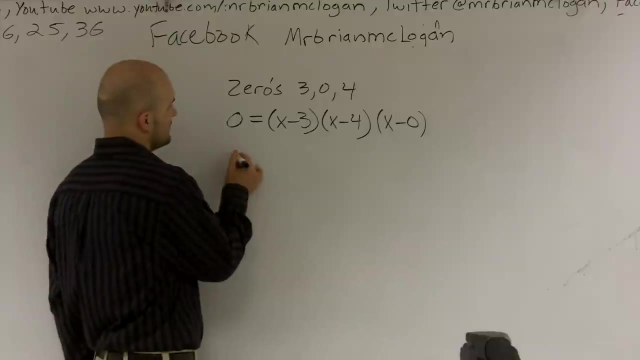 It doesn't really matter. I just changed the order. It should have probably been x and 0 first, But then I'm going to now. I just need to FOIL this out. Let's just multiply it out. I guess I might as well do a little FOIL method. 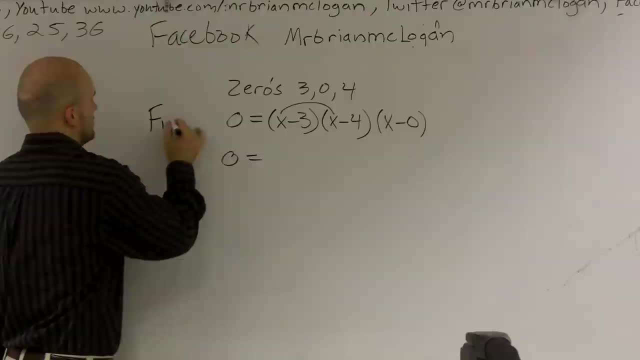 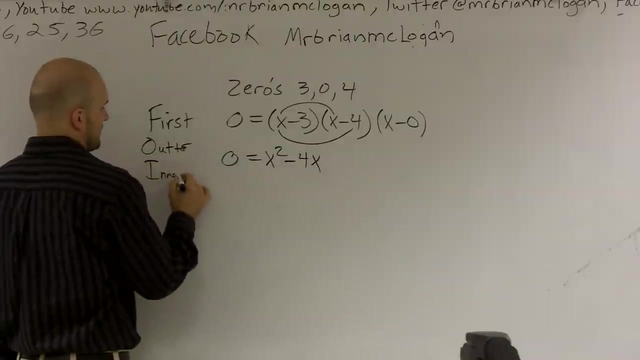 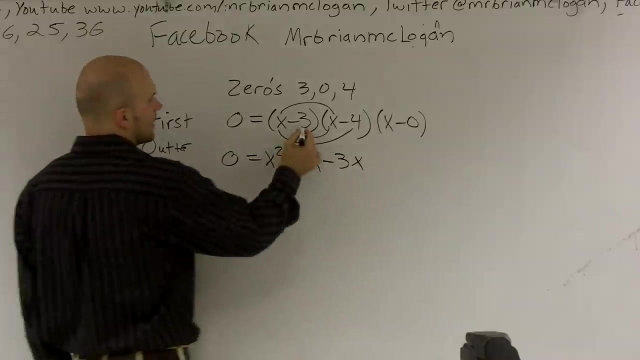 FOIL first right. So x times x is x squared Outer, x times negative 4.. Then you got your inner Negative 3 times x And then you can do your last Negative: 3 times negative, 4 is a positive 12.. 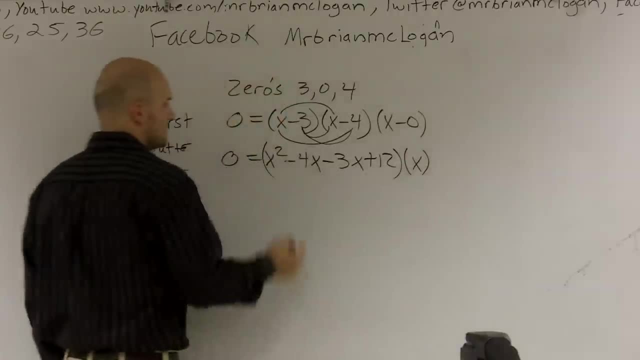 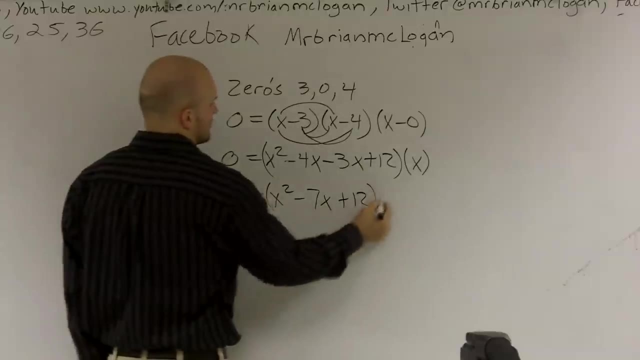 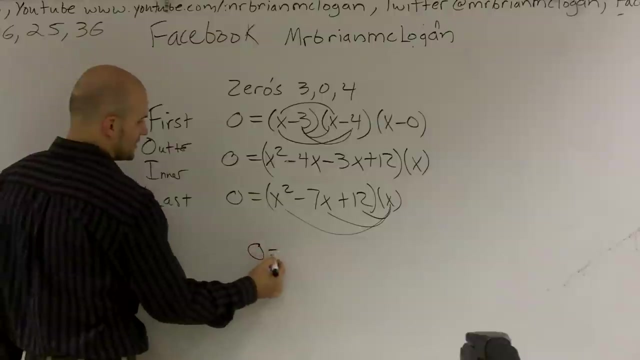 Times x minus 0 is just going to be x, right? I can reduce this to x squared minus 7x plus 12 times x, And then I need to do distributive property with this one, So I get 0 equals x squared. I'm sorry, x cubed. 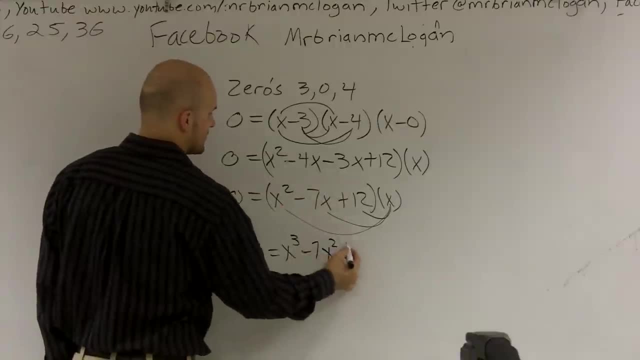 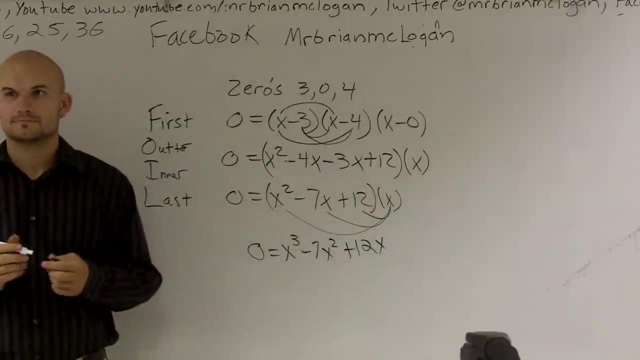 Minus 7x times x, which is a 7x squared plus 12x, And that is your polynomial with those given 0s. That's all you get. Okay, that's all you get. Well, you didn't do subtraction on addition. 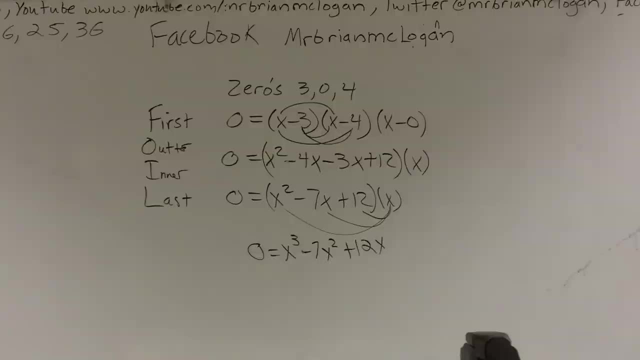 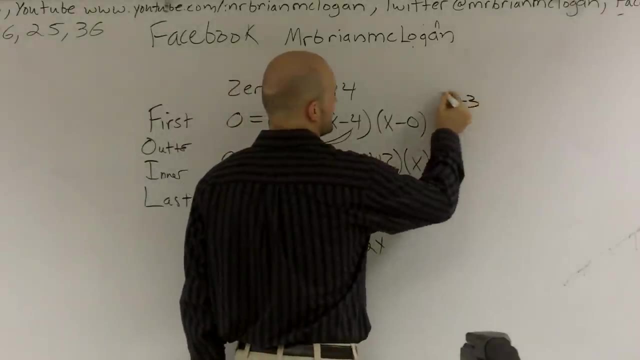 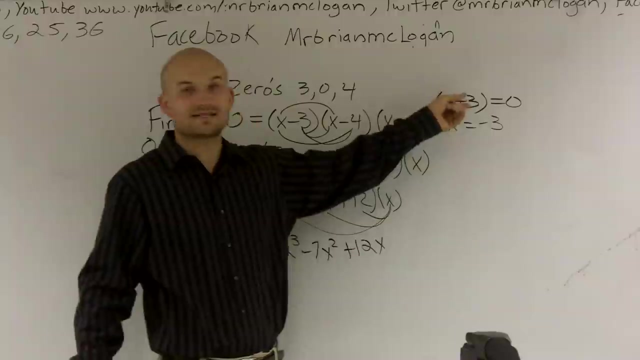 Now you have x minus 3x plus 4, why didn't you do positive? Because if my 0s were x plus 3, then the 0 would be x equals negative 3.. Oh, Remember, if that's a 0,, that's the factor. 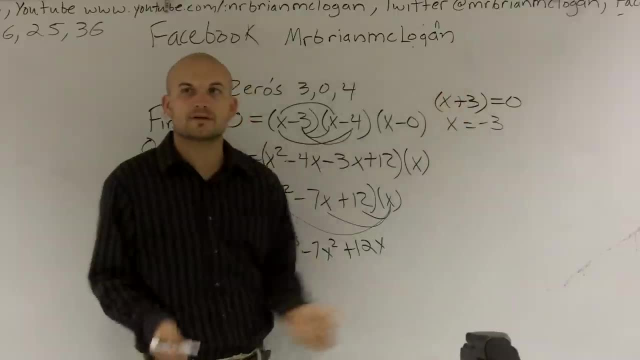 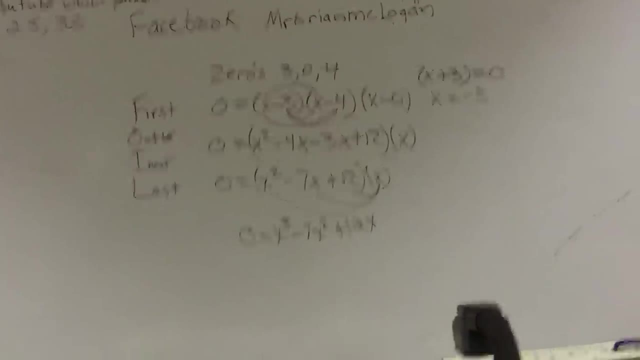